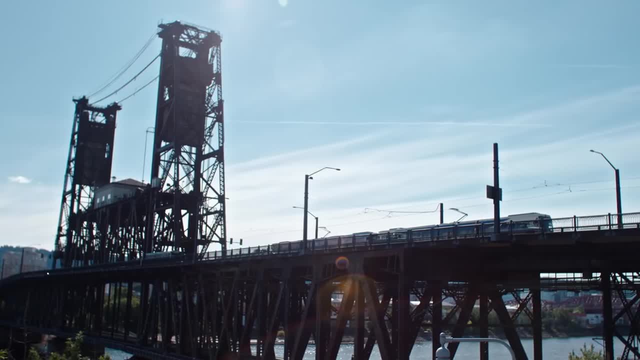 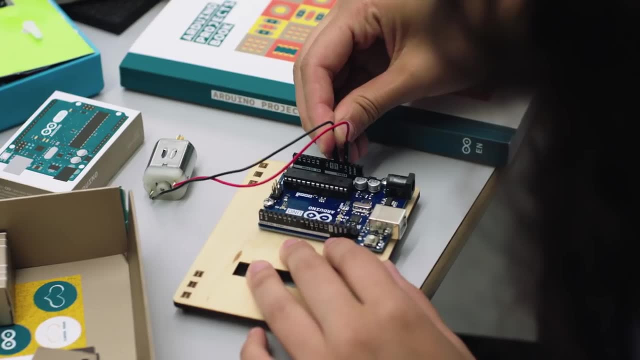 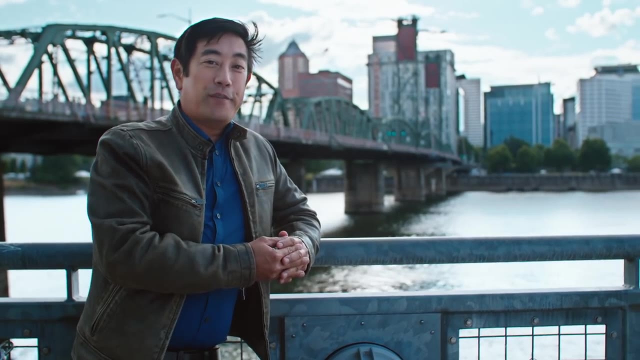 So far on the road to engineering big ideas, we've traveled from the discovery phase to building a working prototype. Now I'm in Portland to explore the crucial next step: refining an initial design to prep it for manufacture. This is Engineering Big Ideas, presented by 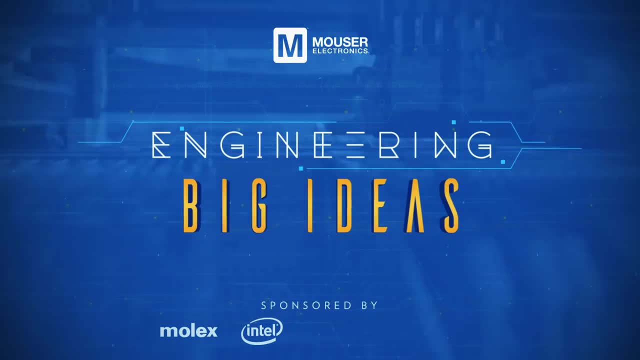 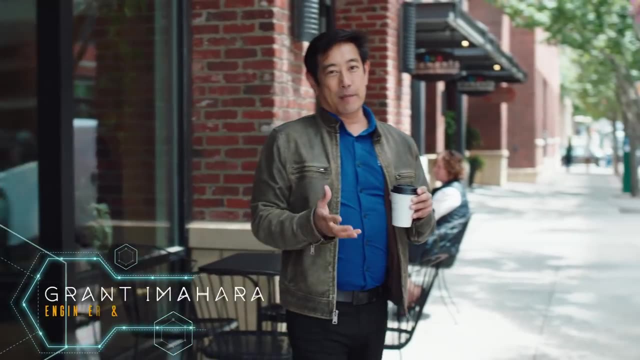 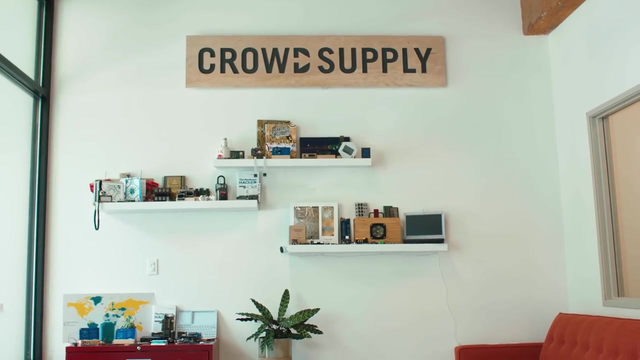 Mouser Electronics, Molex, Intel Analog Devices and Microchip Technology. Refining a concept for manufacture is a critical step in the innovation process, where funding either happens or it doesn't. So let's ask an expert what resources are available to. 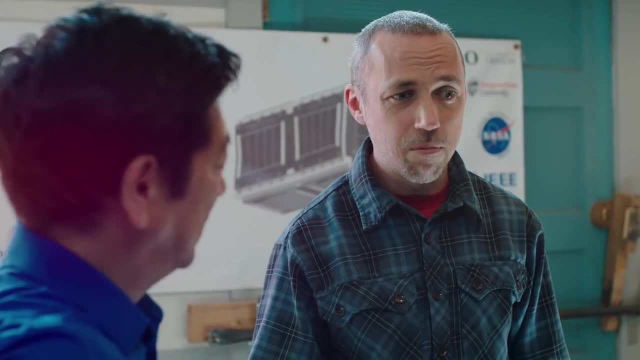 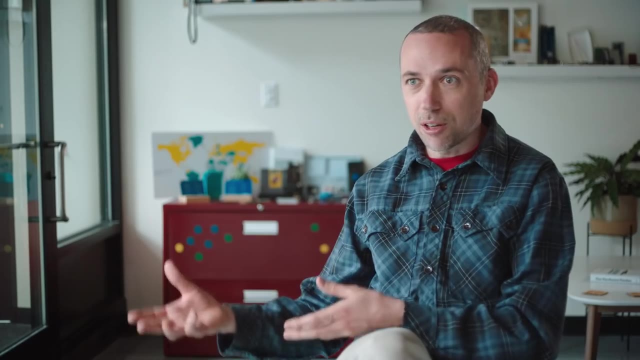 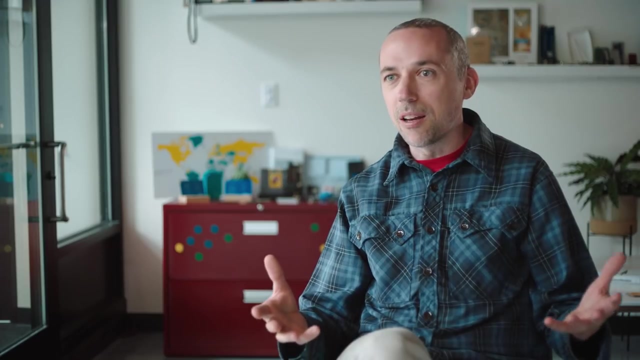 engineers who want to make sure that their concepts actually make it to market. Tell me about CrowdSupply. What do you do CrowdSupply is? It's a crowdfunding platform for electronics right For open source hardware. We help market it to the world, let everyone know about it, and then they place their pre-order, And then 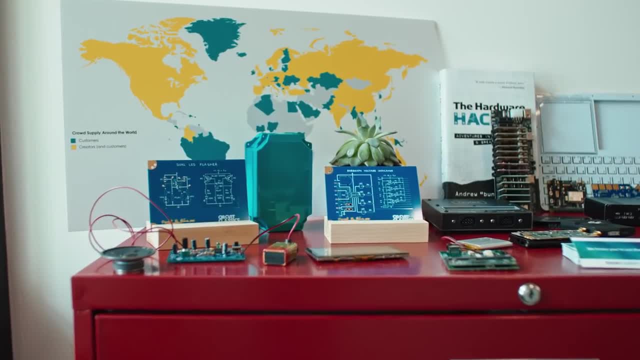 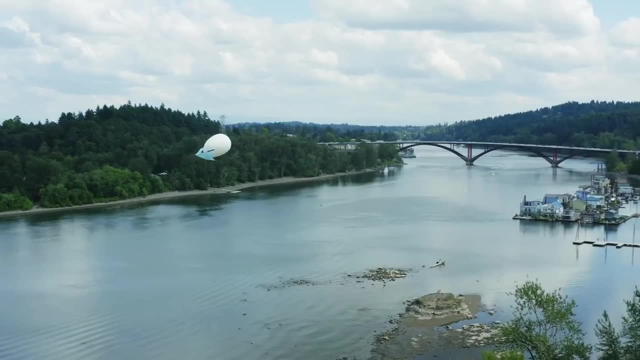 we give the creator that money, they go off and they make it. This is a risk mitigation strategy. You don't want to make 10,000 of something when they find out nobody wants it. This is the AirPup. It is a kite balloon. 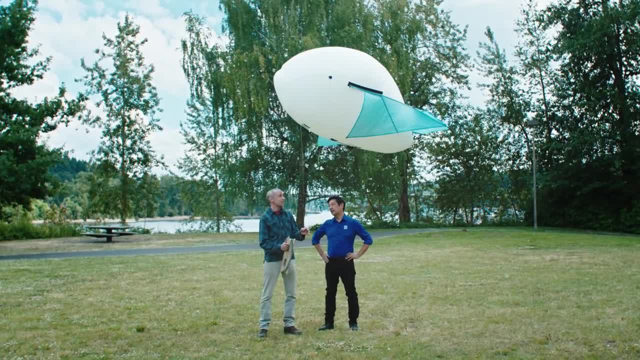 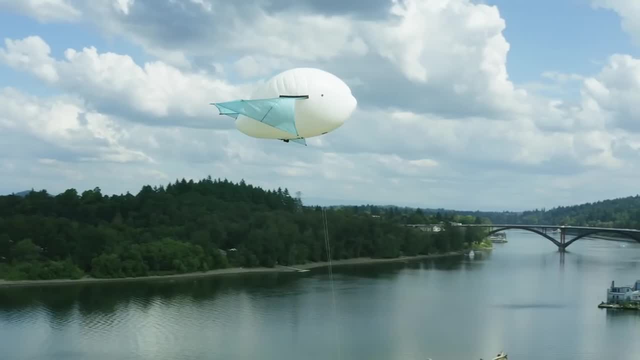 Okay. So it's a helium-filled balloon, but it has the aerodynamics of a kite. This would go anywhere where a drone wouldn't be able to go. You know, if you needed it in the air for, say, three days at a time instead of 15 minutes, you'd send this, Or? 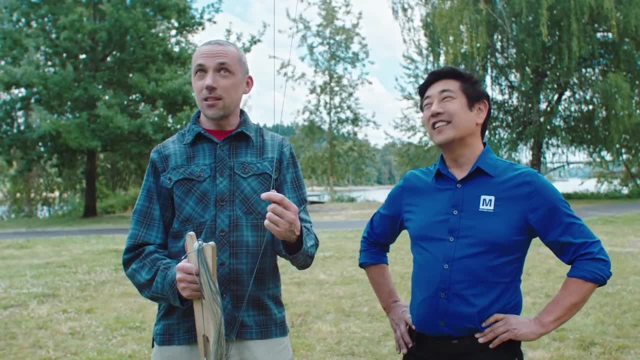 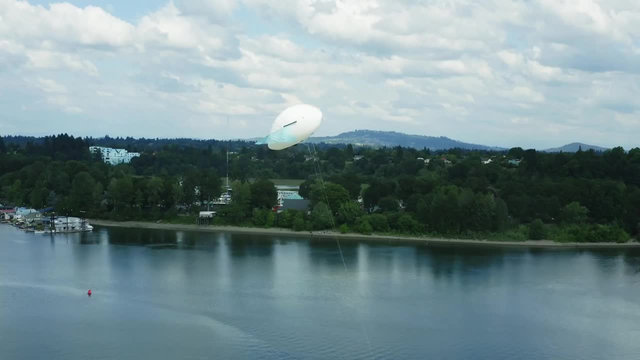 it has to be quiet, Sure, Or It's totally passive. Passive, yep, There's no motors on it. It does have a payload there, as you can see. You know the camera is on there. You could put weather sensors or other things on there. 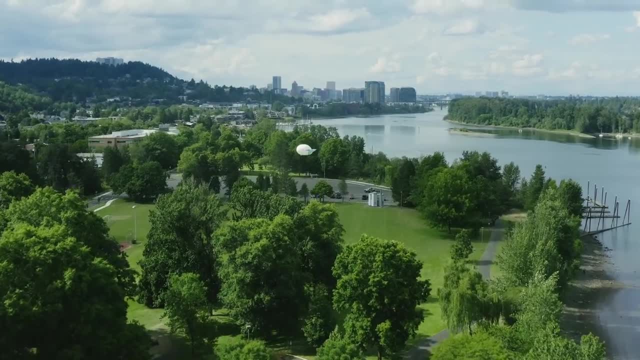 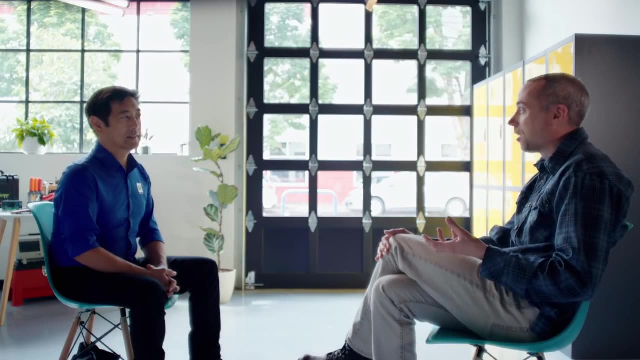 too. Now we're seeing kind of a second-generation product coming out of technology that was born at CrowdSupply. There's tens of hundreds of thousands of people out there with a drone, So it's a great platform. Yeah, There's a lot of people out there with product they got at CrowdSupply. We're interested. 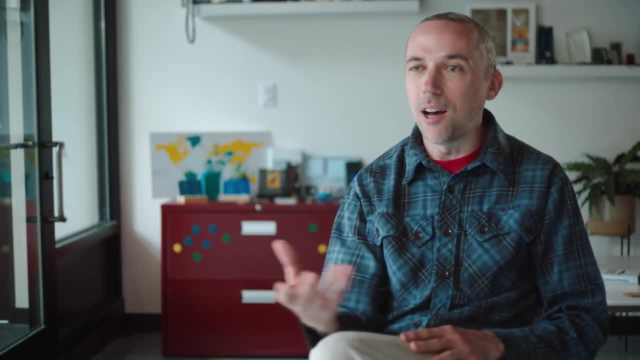 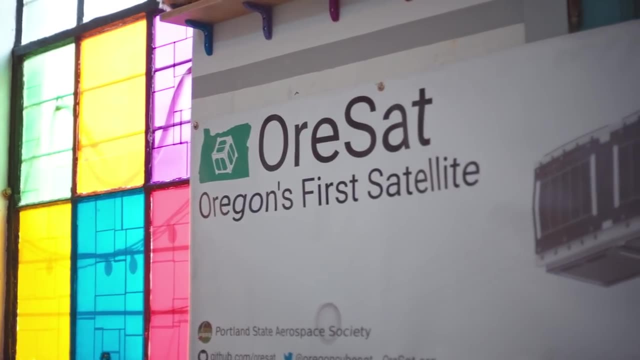 in finding out what those people are doing, What prompted them to buy this new product and what are they doing with it now and what is it turning into Right? The ORSAT project is a good example. They got a LIME SDR and now they're making a satellite.